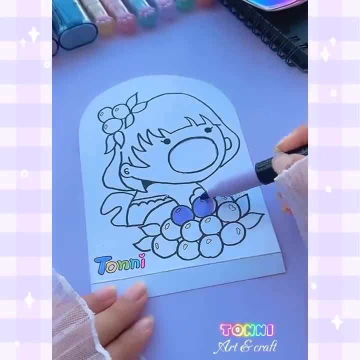 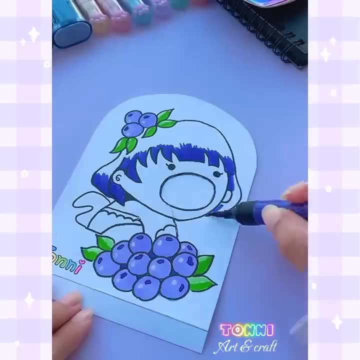 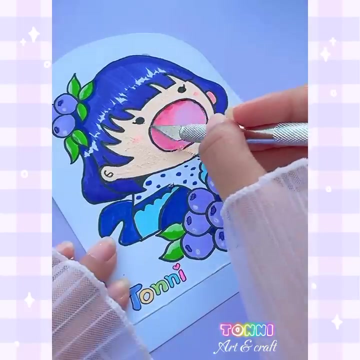 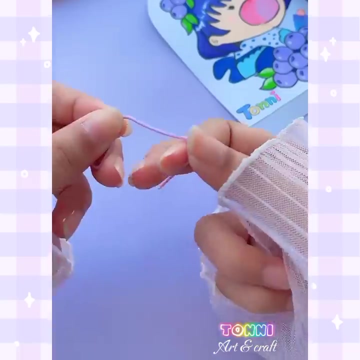 We don't need to rush, cause I got forever. What is meant to be is gonna be. It's you and me. that's what I believe. I won't give up. I'll keep it up until it's over. I know it's gonna take some time, But I won't make you mine. 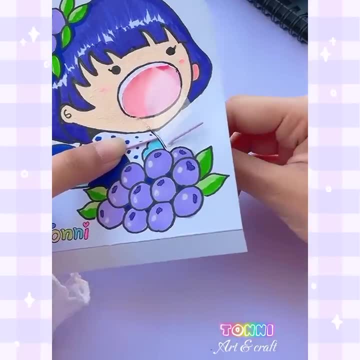 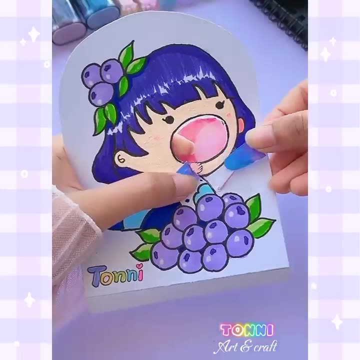 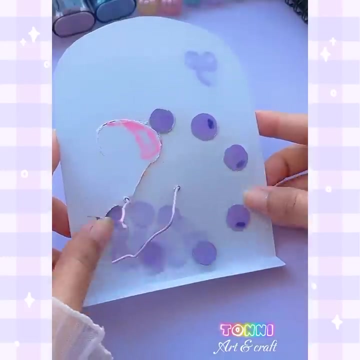 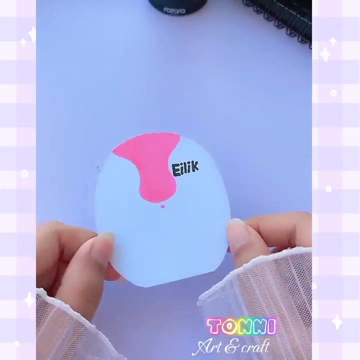 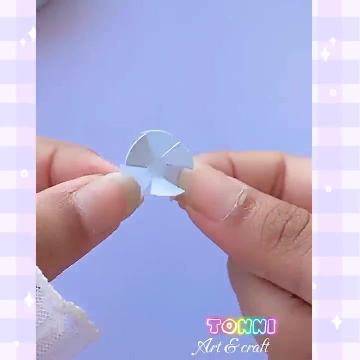 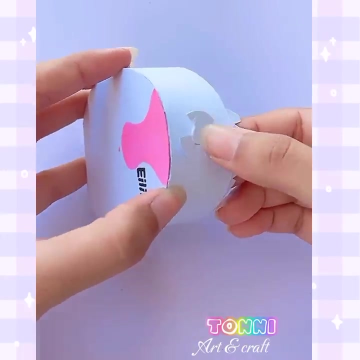 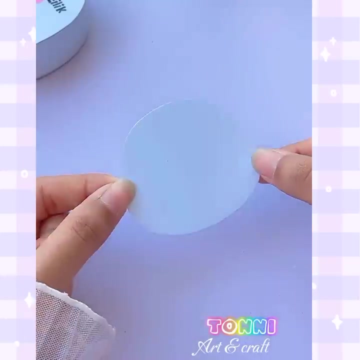 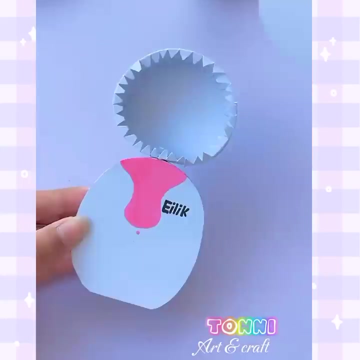 I'll go the extra mile. I'll do what needs to be done Until the race is won. I'll go the extra mile. Until the race is won, I'll go the extra mile. Put your faith in me and let yourself believe That I'm all you need. I'm all you need. 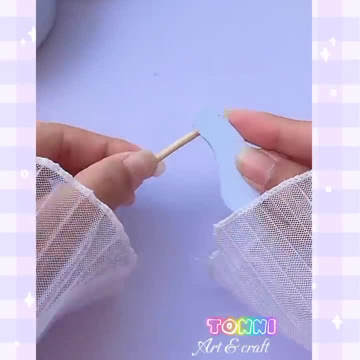 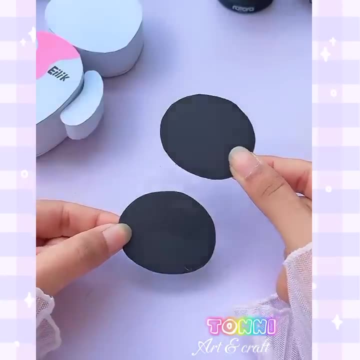 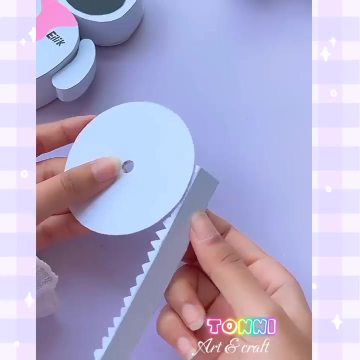 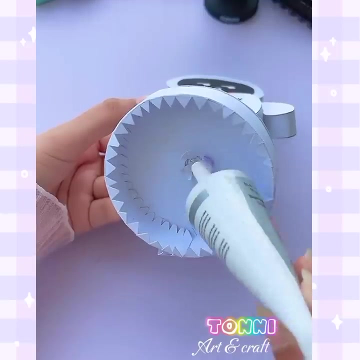 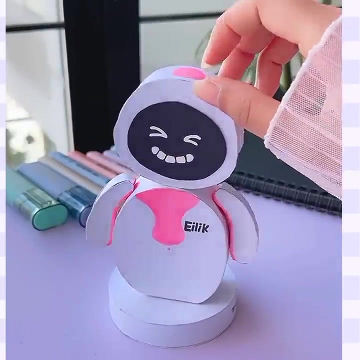 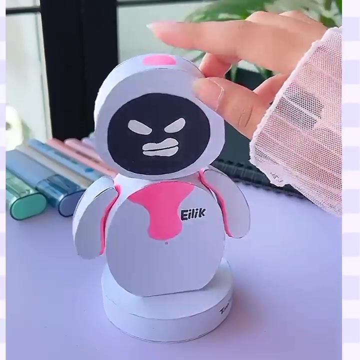 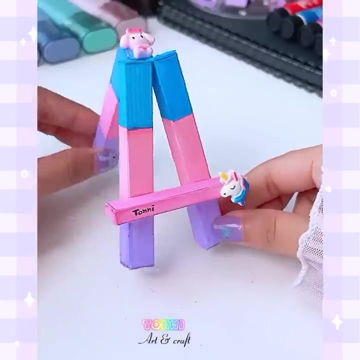 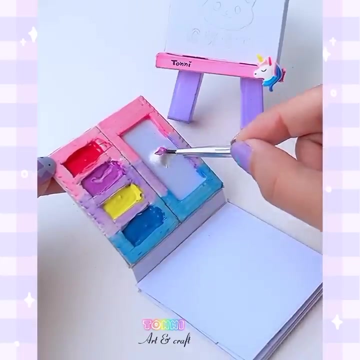 I'll make you see that it's you and me, you and me. I'll do what needs to be done Until the race is won. I'll go the extra mile, Go the extra mile. Just watch me, just watch me, just watch me. I won't make it easy for you now. 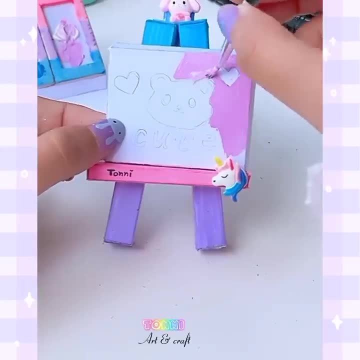 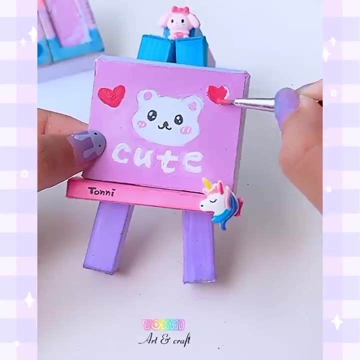 You got two minutes of my time And I don't really break too easy, But I'm worth it, cause I'll slip into your dreams tonight, oh. So give me, so give me your all, I'll take it. I'll take it to Mars, oh. 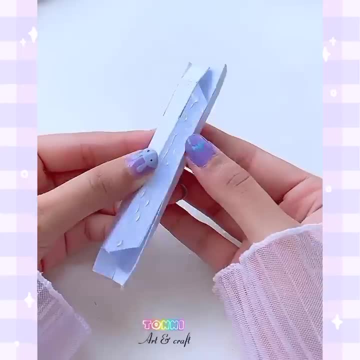 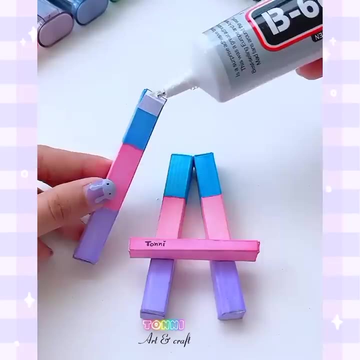 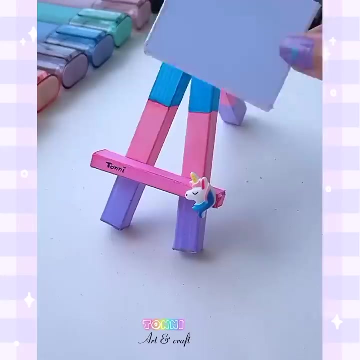 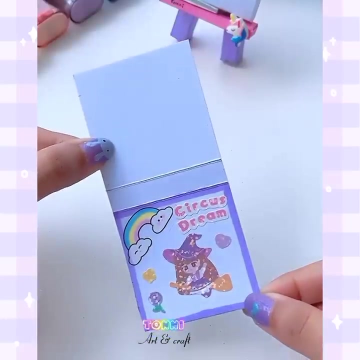 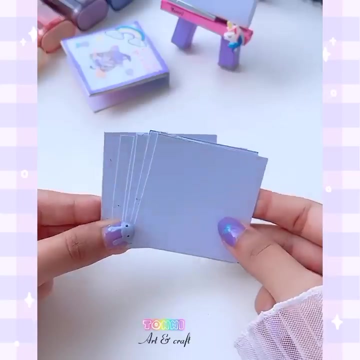 I'll stick like glue inside your mind. So give me, so give me your all. I'll take it. I'll take it to Mars. oh, I'll stick like glue inside your mind. Just watch me. I got you wrapped around my finger, But don't you ever let me go. 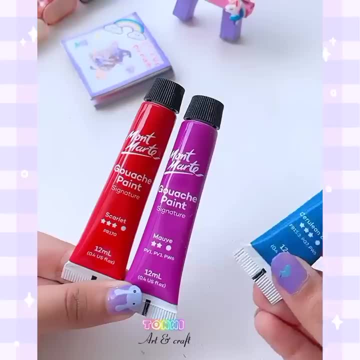 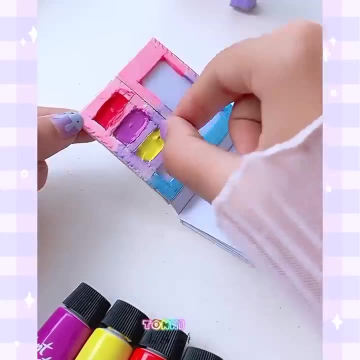 But don't you ever let me go. But don't you ever let me go. Don't you try to call me tomorrow. There's nothing personal in having a little fun. You'll wait and see if it's worth your while. So give me. so give me your all. 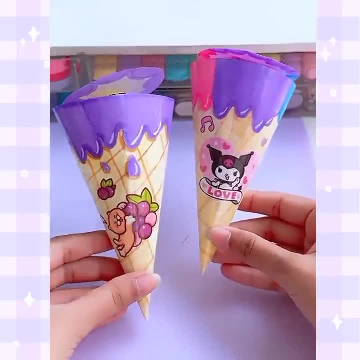 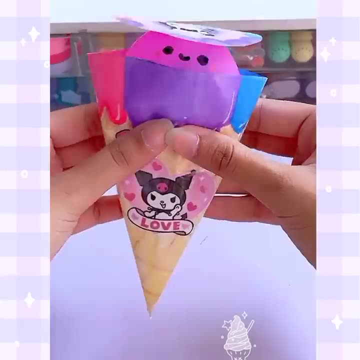 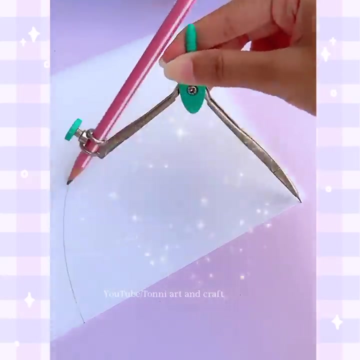 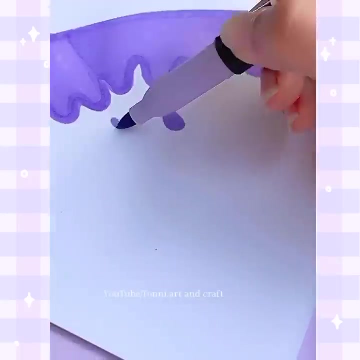 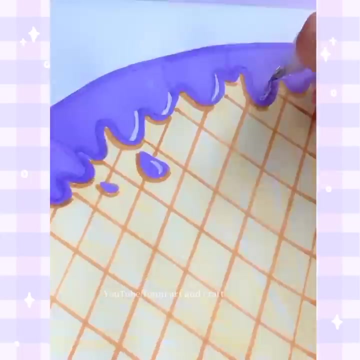 I'll take it. I'll take it to. We fell in love at a bad time, Getting insecure, Questioning myself on the way down. Now I'm so tired of breathing on the water, I just wanna flow like a ship Made out of paper. Right now I need to. 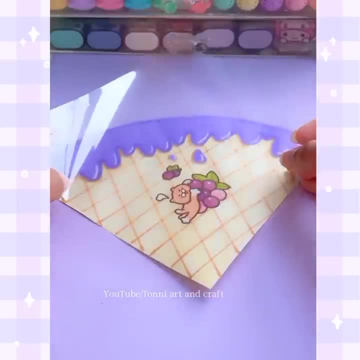 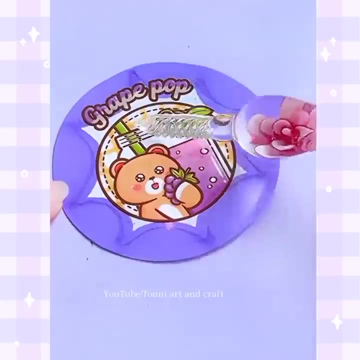 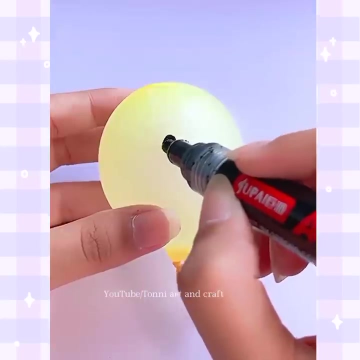 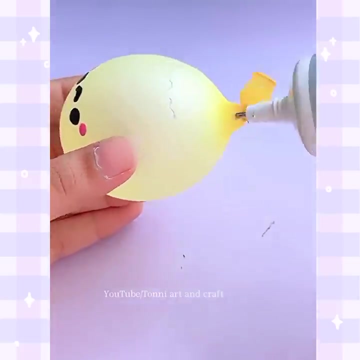 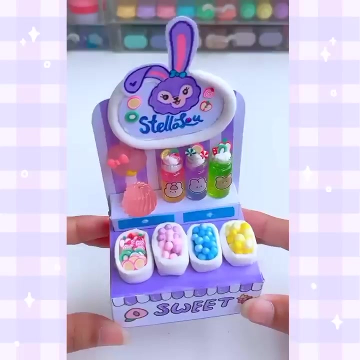 Take care of myself, Comforting myself Like a roller coaster. One week I am. One week I am. Oh, next one I'll be down, But I'm getting closer to A stronger me Feeling free Like a roller coaster. A stronger me Feeling free Like a roller coaster. 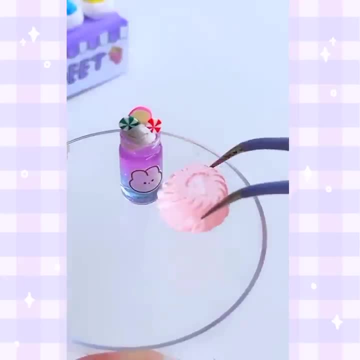 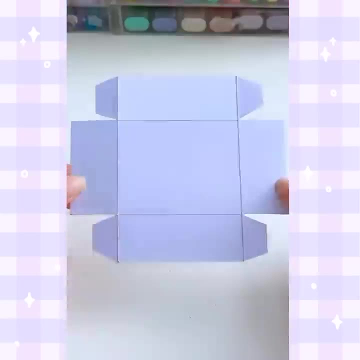 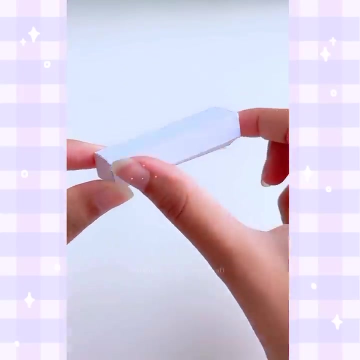 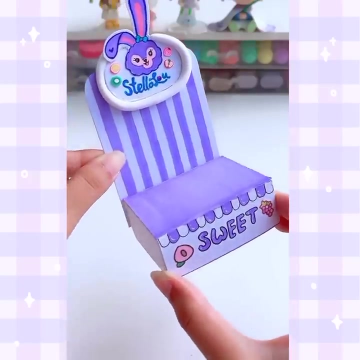 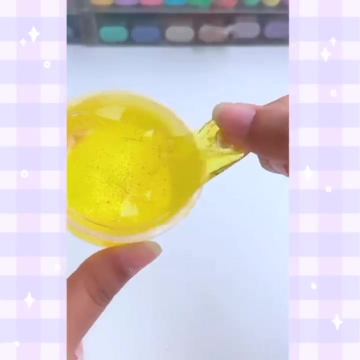 Grandpa used to ask Why I'm single with such a pretty face. Where is your man? You should go out and chase him Now. I'm so tired of breathing on the water. I just wanna flow like a ship Made out of paper. So now I'm about to. 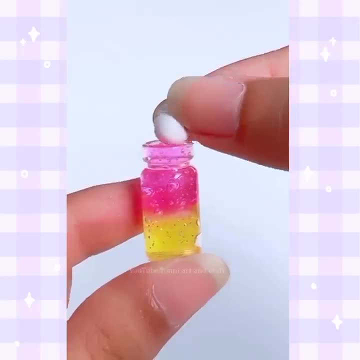 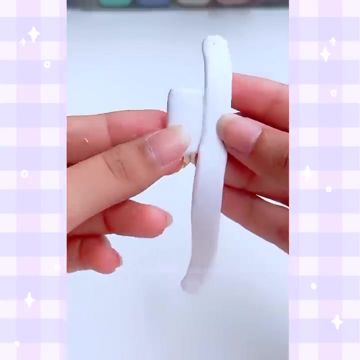 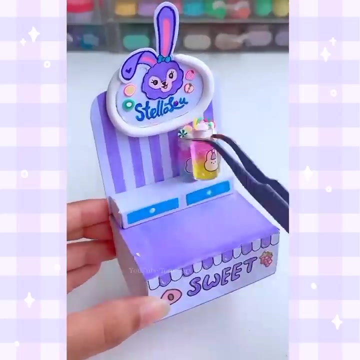 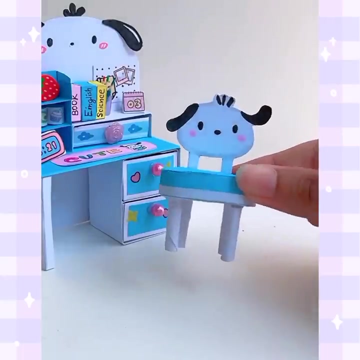 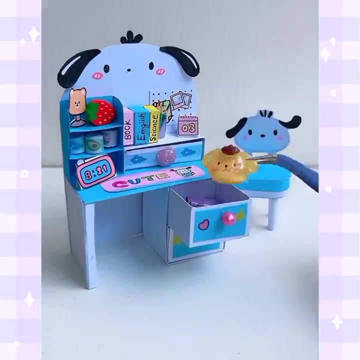 Take care of myself, Comforting myself Like a roller coaster- One week, I am. One week I am. One week I am. Oh, next one, I'll be down. But I'm getting closer to A stronger me Feeling free Like a roller coaster. A stronger me Feeling free. 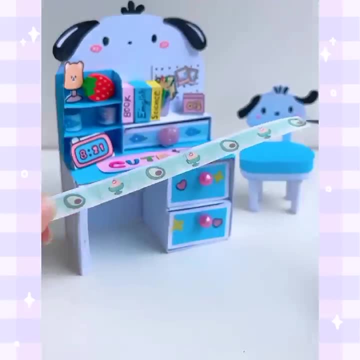 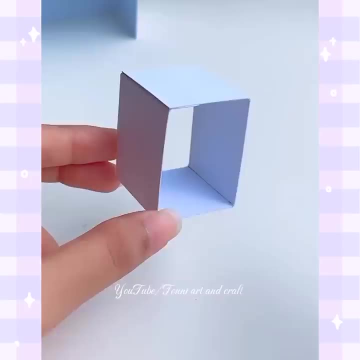 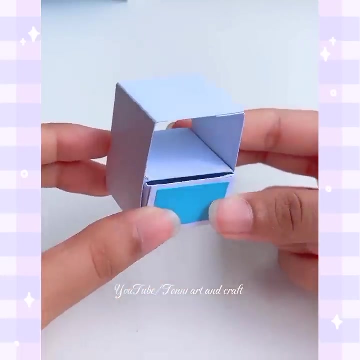 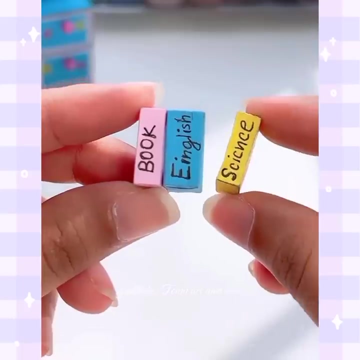 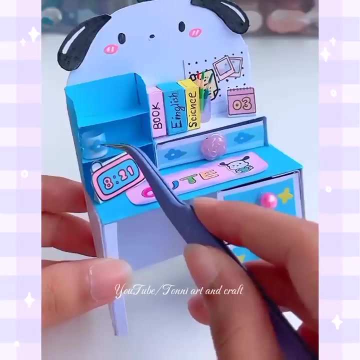 Like a roller coaster. Don't need anyone else, I just wanna be for myself A while. nobody else, I just need myself. Take care of myself, Comforting myself Like a roller coaster. One one week I am up, Next one I'll be down. But I'm getting closer to. 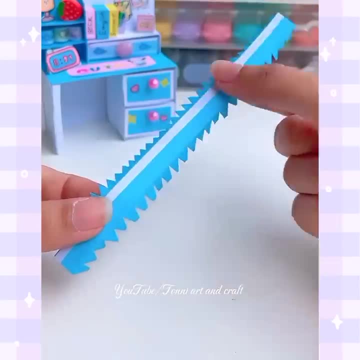 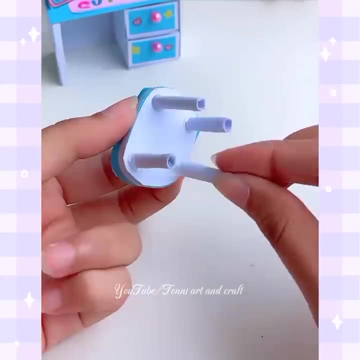 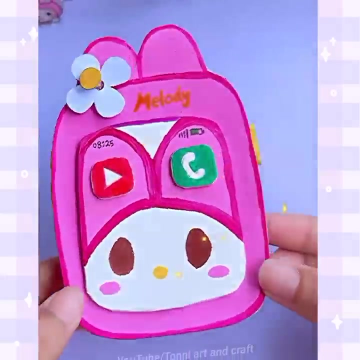 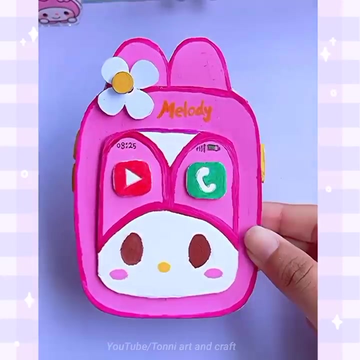 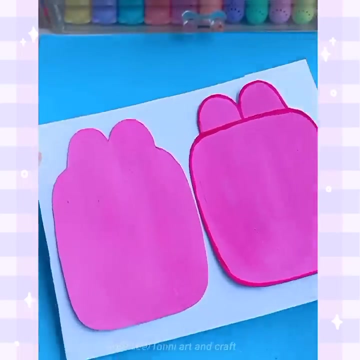 Stronger me Feeling free Like a roller coaster. Stronger me Feeling free Like a roller coaster. Always my own damn fault That I've fallen for you. We haven't even talked. Still, I'm obsessed With you. Was it your milky eyes Or your skin, I don't know. 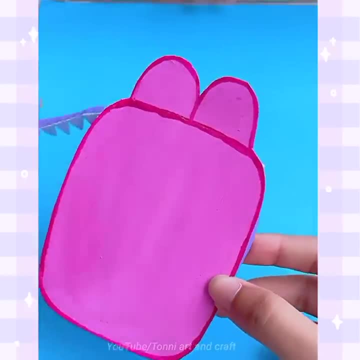 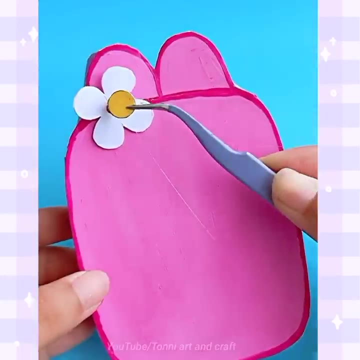 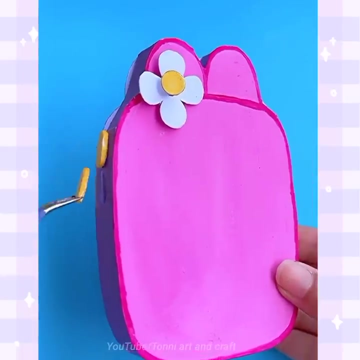 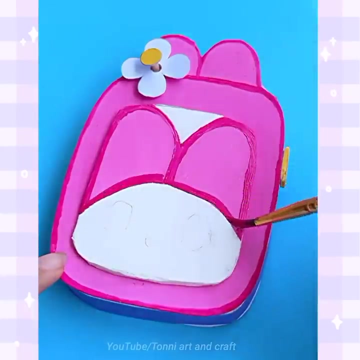 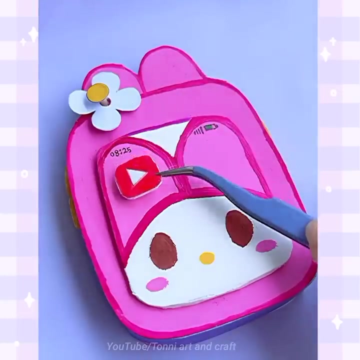 Doesn't matter anyway, Cause I'm never letting you go. I know It's Gonna take some time, But I won't make you mine. I'll Go the extra mile. I'll Do What needs to be done. Until the rays is one, I'll Go the extra mile. 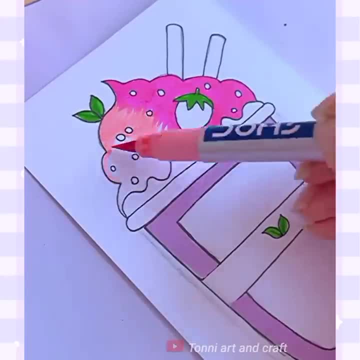 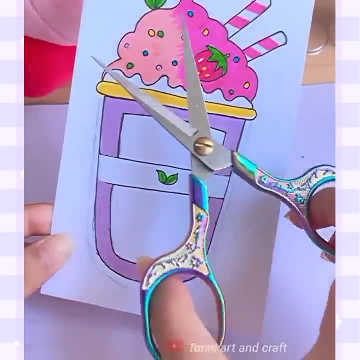 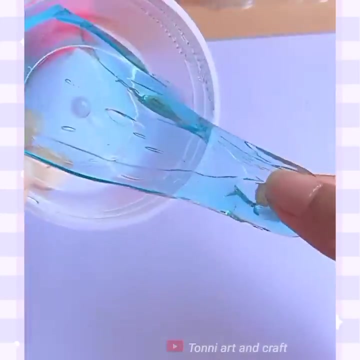 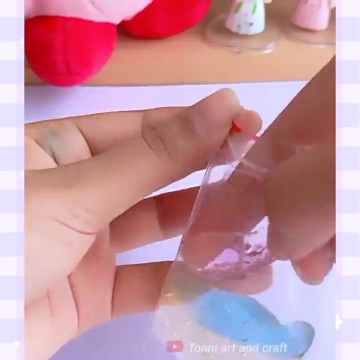 If you don't love me Now, you will love me later. We don't need to rush, Cause I got forever. What is meant to be Is gonna be. It's you and me. That's what I believe. I won't give up. I'll keep it up Until it's over.